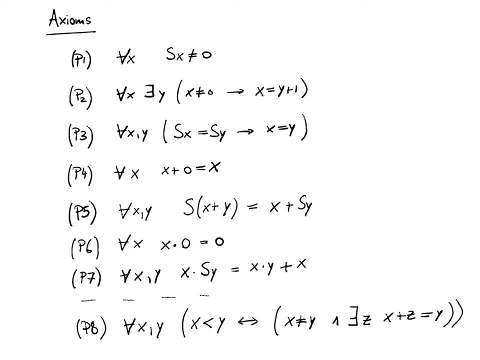 among non-negative integers. So for example, for every x, here the successor of x is not equal to zero. for every x, every y, if x is not zero, then it has a predecessor, and of course here. now you see I already slipped back into the other in the old notation, so this should of course be s of y. 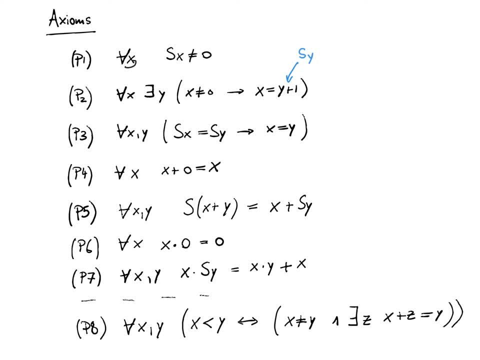 all right. and then the next one: if two successors of are the same, then the numbers are the same. and then addition. here those two next axioms actually say that addition is. so the addition symbol or the function given by addition is obtained from the successor operation inductively right. so if you 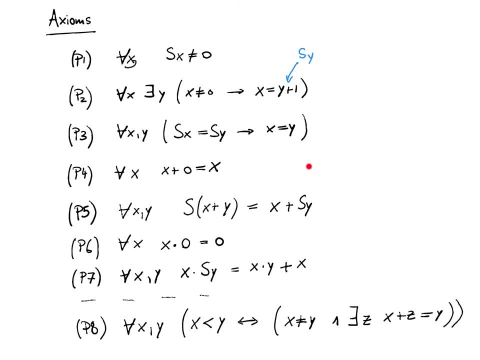 look at these two axioms together. this is just the recursive definition of addition and this, these two axioms, tell us that addition has to be related to the successor function in this way and similarly for multiplication. so p6 and p7 essentially just tell us that multiplication is. 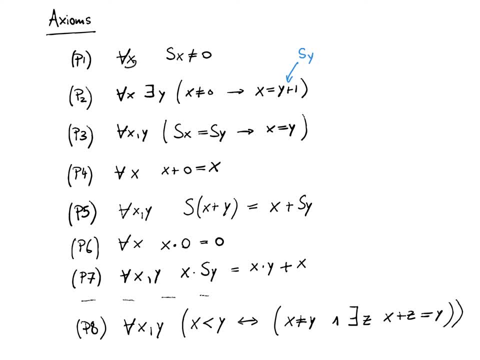 obtained recursively from addition. so these seven axioms together actually have a name. they're also called q after robinson's, or robinson's q, and the important fact here is that this is a finite theory, so there's only finitely many axioms now. the axiom p8, as i already mentioned before, is just ensuring that less than is an expansion by 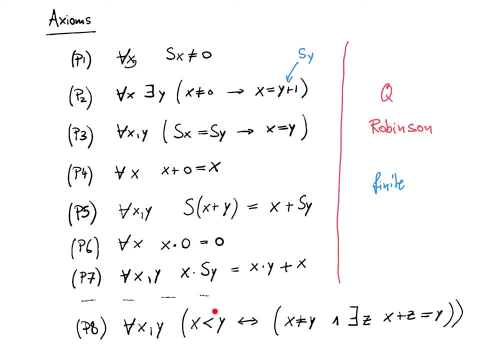 definition, because we can define less than using the other symbols of the language using this formula here. so in the following way, let me just put all of this together because this is just a measure of the number of axioms we want to use. let's use a lot of examples and I hope this will help you and I'm happy to answer some of your questions if you have other questions in the future. so if you have any questions, you can just put those in the comments below. 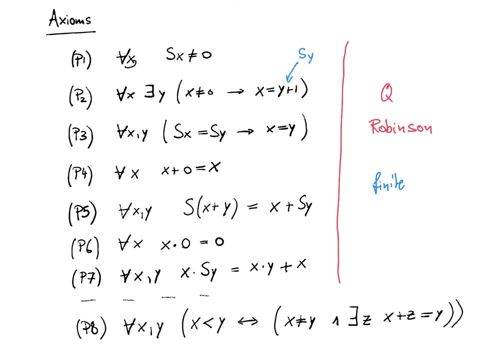 right using this formula here. so in the following way of having the values T instead of the other symbols we want to use. so in the following way of having the values T instead of the other symbols we want to use, we will denote the theory that we obtain by adding P1 through P8.. So all of these, 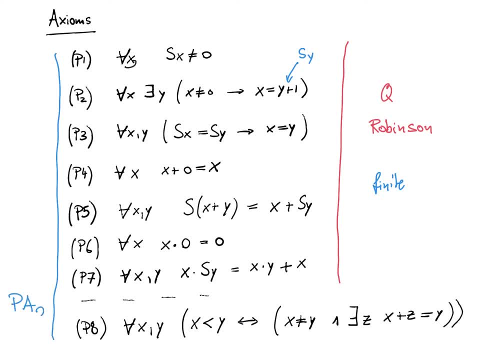 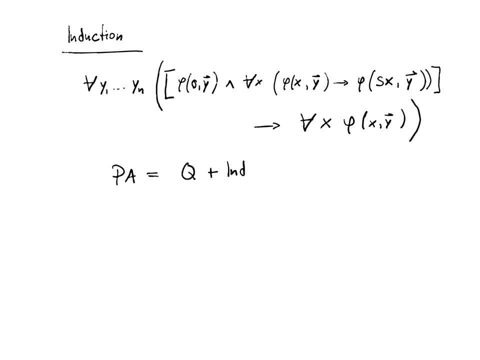 axioms together, this will be PA0.. But since PA0, so P8 is just an expansion. by definition, it cannot prove more than Q, so it's really the Q is the core of this. So Q is a finite theory, but it is actually quite weak as we will see It. 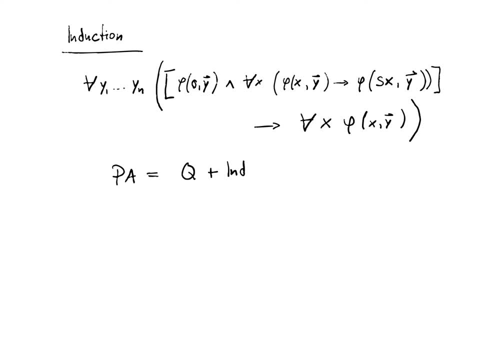 just captures some very basic facts about arithmetic. To get full PA we have to add the induction axiom, which is really not an axiom but a scheme, because we have to add for any formula right, so for any formula phi, for any phi. 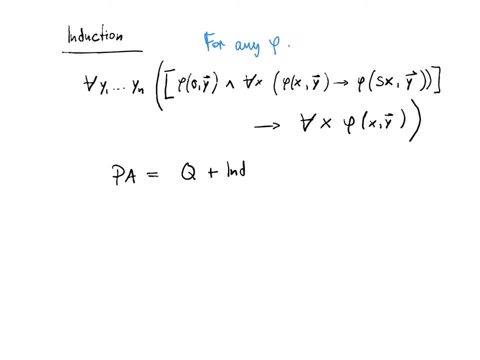 right. so for any formula phi for any phi. right. so for any formula phi for any phi. this is an axiom, so let's call this int phi. And if we add these infinitely many axioms of this form, for any formula, we add one. so there's. 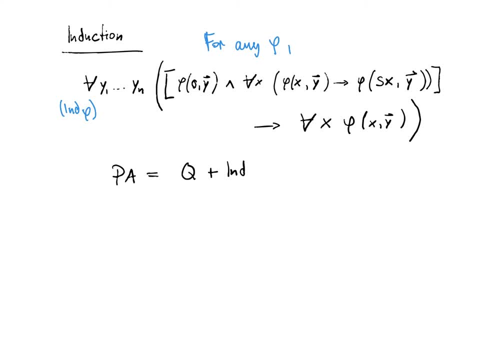 infinitely many formulas, so we have to add infinitely many formulas. If we add this to Q, we get the theory of Peano arithmetic. So this is not a finite theory anymore. So we have the following relation between the different theories: Clearly Q is a subtheory of PA, but Q, as we saw, is finite and therefore 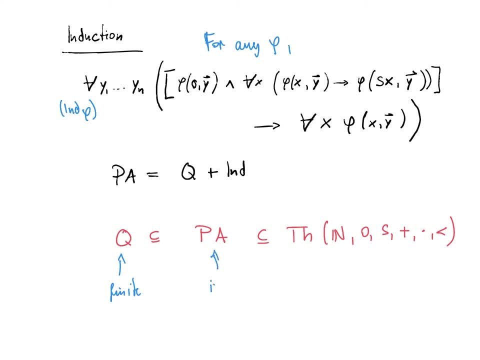 recursively axiomatizable. PA is infinite, but still recursively axiomatizable because if you, you can check whether a formula is of this form. So we have a still recursively axiomatizable theory And of course both are subtheories of the theory of the natural numbers. 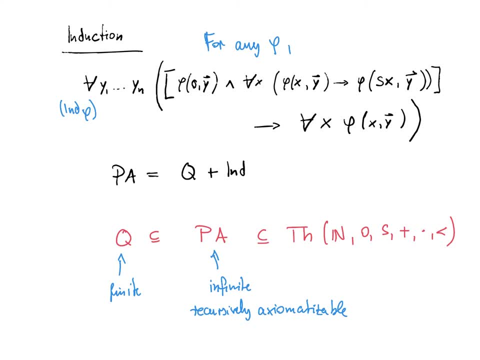 because all of those statements hold in the structure of the natural numbers. So, in particular, every sentence in PA is a true statement about the natural numbers. So this is infinite, of course, And, as we will see, the theory of the natural numbers is not decidable. 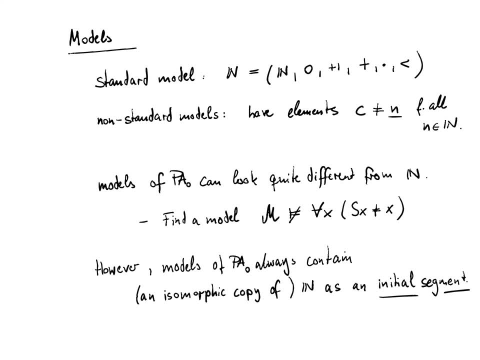 Now, what do models of Q or PA0 look like? Of course, we always have the standard model of the natural numbers, But, as we have already seen from as an application of the compactness theorem, there are also non-standard models, And non-standard models are those that have elements that are different. 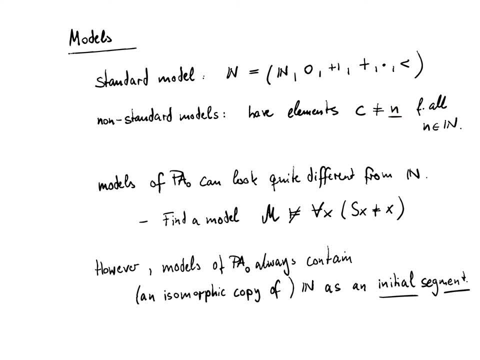 from the interpretation of this constant symbol, n for every n in n. Models of PA0 can also look quite differently from n. So as an exercise, I encourage you to think: see if you can find a model of PA0 or Q which that this doesn't hold. 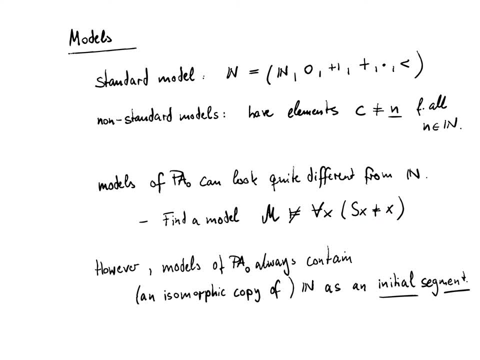 So for all, x, the successor of x, is different from x. However, there's one important fact that will be actually quite important for us about models of PA0. Namely, they always contain an isomorphic copy of the natural numbers as an initial segment. 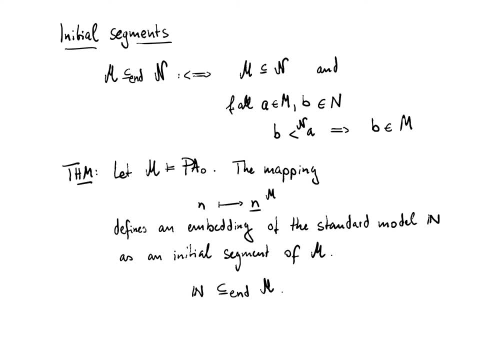 So what exactly is an initial segment? Probably you have already a good idea, But let's look at the formal definition. So two structures. we say n is an end extension of m And correspondingly m is an initial segment of n. 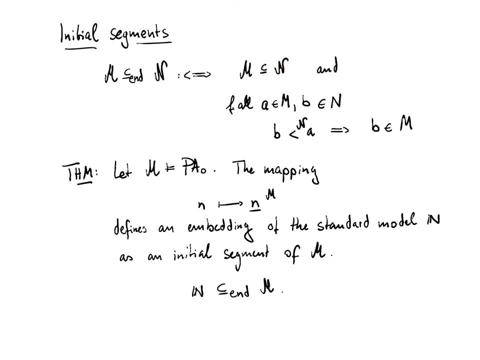 If, and only if, m is a substructure of n And for all, a in m and b in n. if b is in n below a, then it's already in m in the smaller structure. So there's nothing between the elements of m in the bigger structure n. 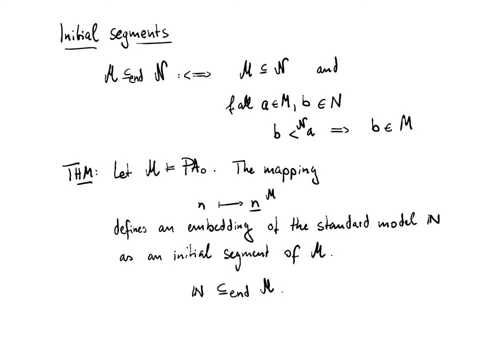 And the theorem is that if we have a model of PA0, then the mapping that maps the natural number n to the interpretation of the constant symbol n in m, that defines an embedding of the standard model n as an initial segment, In this sense here, of m. 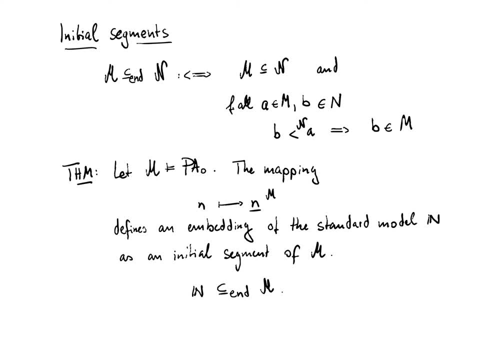 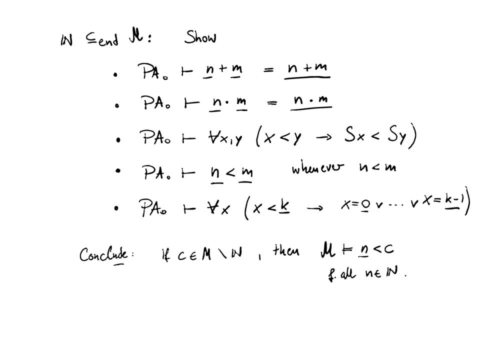 So, in other words, n is an initial segment of m, m is an end extension of n. In order to prove this, you have to kind of go through the following steps, And of course I encourage you to do that. First, you show that addition and multiplication defines a homomorphism. 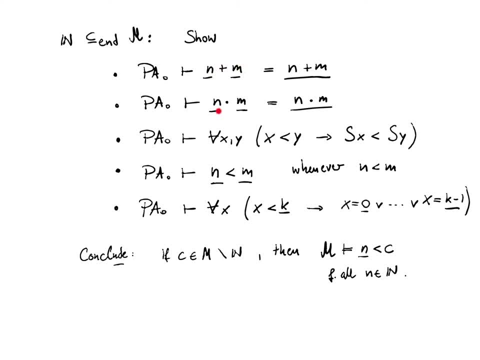 of the structure when restricted to the interpretation of the constant symbols. So our mapping that we're interested in, namely mapping n to interpretation of m in m, that will be in homomorphism. So how do you prove this? Well, you do it by induction. 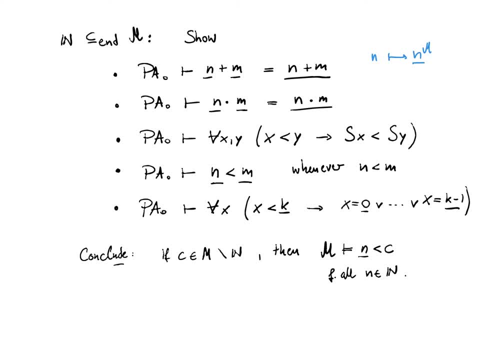 So now you will say: well, wait, don't we lack induction in PA0?? Yes, we lack it in the theory itself, but we still have it in the meta theory And, as you see, we don't show this in the form of for all n or something. 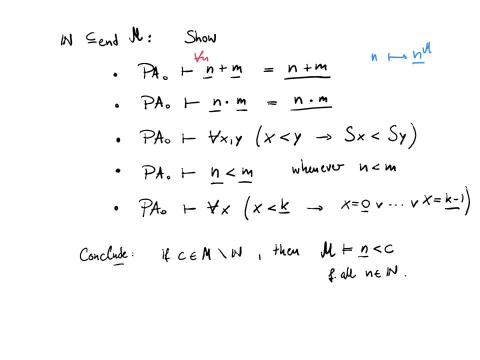 So we don't show like for all n or something like that. Right, This is an individual statement, right, about a single instance for two numbers or two constant symbols, And this you can show using induction in the meta theory. So induction on n. 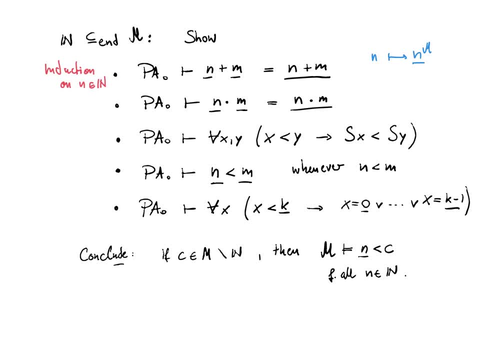 where n now is an element of the natural numbers. You can think of this as maybe naive induction, or induction in the meta theory, And, as I said, this is a single statement, right? And then, once you have proved, once you have showed this, this holds for one n. 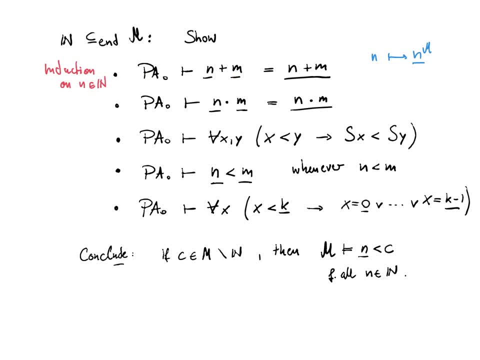 then you move on to the next n, and so on. You don't show a for all statement here. Next, you use the axioms to show that the less than relation is preserved under successor, And this. so for this you use the axioms.